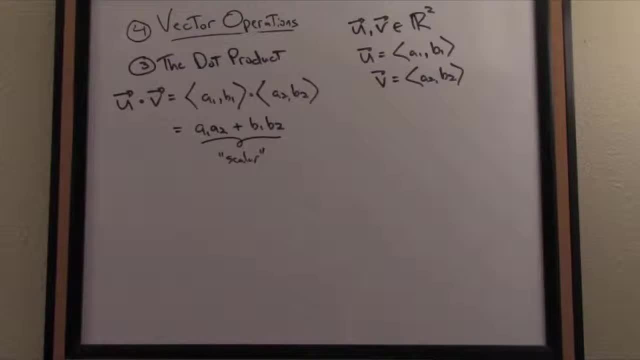 Right Added together so that results in a new real number, In other words, a new scalar. Another natural question to ask is: well, how would I extend this definition into higher dimensions? So, in other words, if I had two three-dimensional vectors and I wanted to perform the dot product? 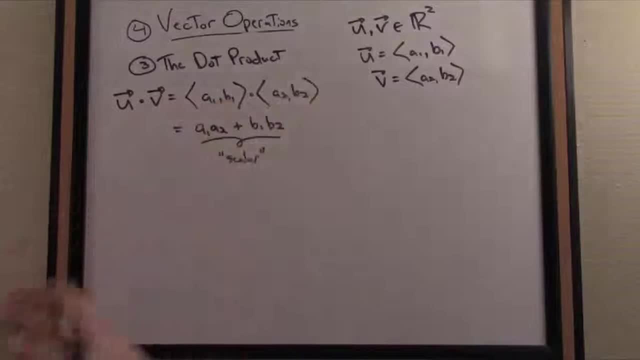 I would multiply the x components together, the y components together and then the z components together and take the sum of all those products. That would give me the result of the dot product, which is once again a scalar and so forth for higher dimensional vectors. 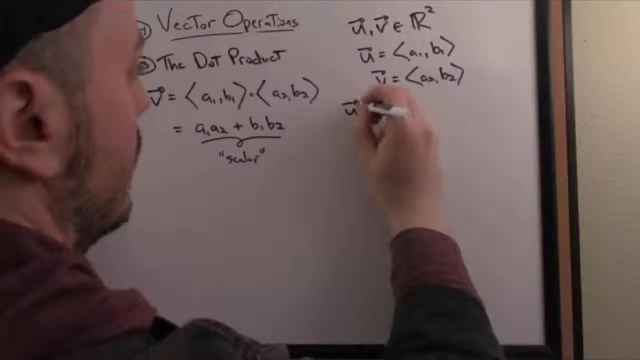 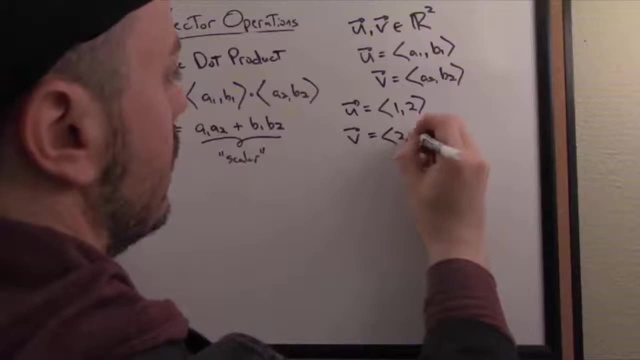 Okay, so let's do a quick example, numerical example, just to kind of see that in action. So if I have the vector u and the vector v, let's just use some of those same vectors we looked at last time, and I want to 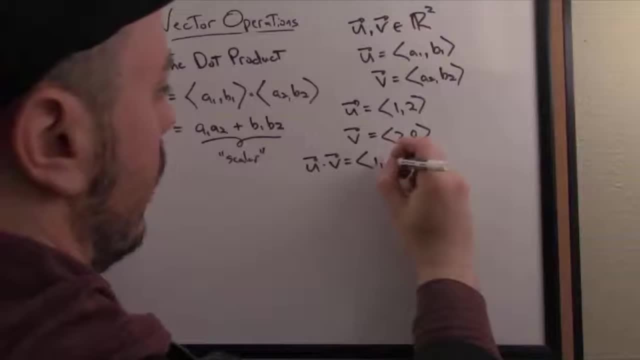 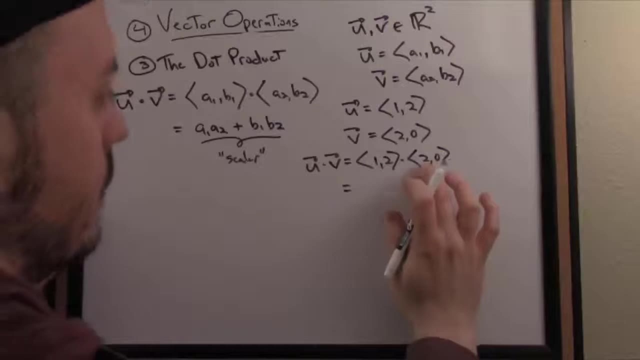 calculate the dot product of those two vectors. I would then say 1, 2 dotted with 2, 0.. Okay, and I multiply the components together. x components first. 1 times 2 is 2, and I add to that the product of the y. 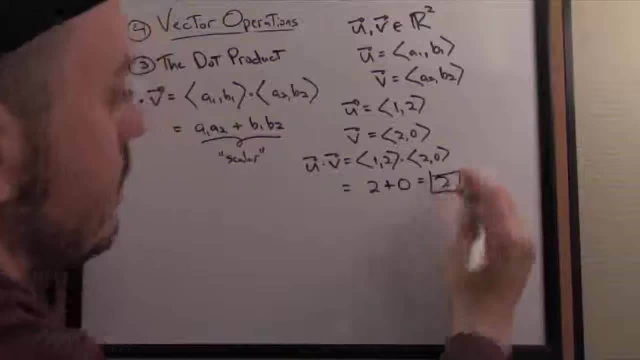 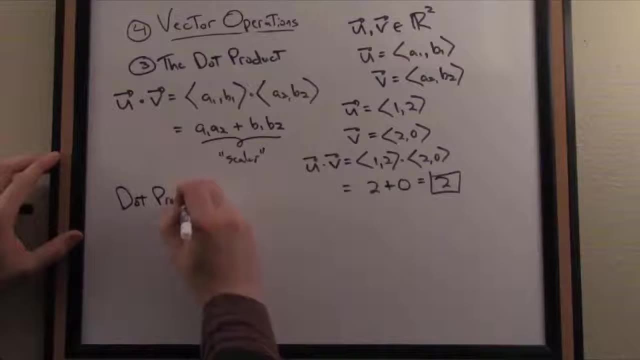 components and I get 0, so 2 plus 0 is 2.. Notice: there is a scalar value for my dot product. The dot product geometrically introduces angles, as we'll see in a moment, and also magnitude or the length of a vector. 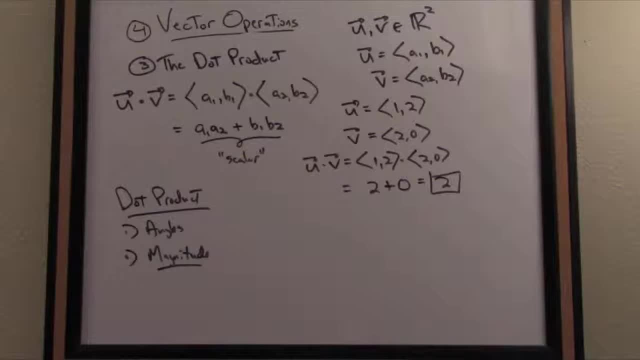 Okay, let's discuss magnitude for a second and how it relates to the dot product. Well, the magnitude or the length of the vector, Let's see. how would I define this? Well, first off, start with our vector. 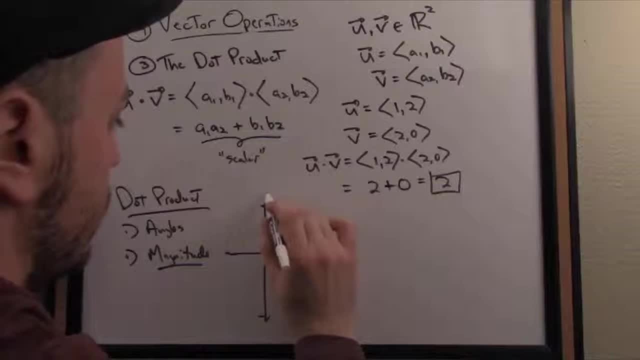 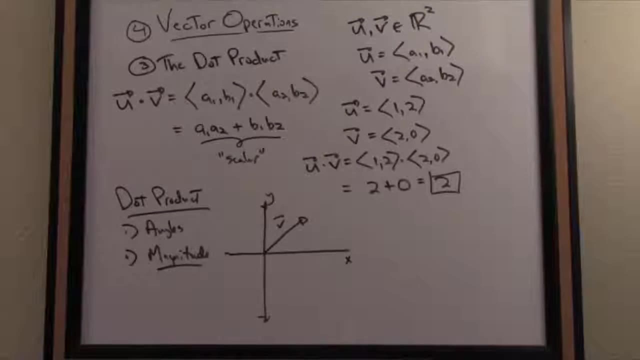 again, v, let's say in the plane And let's say v, consists of those components as I've written it before, And the notation here for the length or the magnitude. it's also called the norm of the vector most commonly. 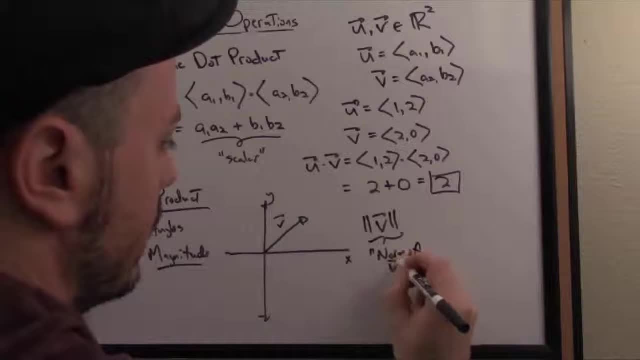 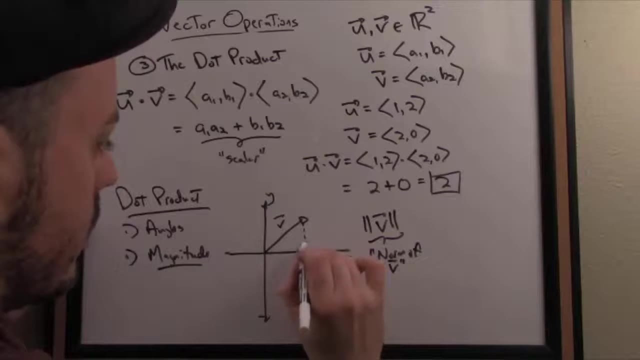 So you would say the norm of v, which is just a number meaning the length of the vector v, the norm of that vector. how do I find that algebraically? Well, I can think of drawing a right triangle here, and let's say the components. 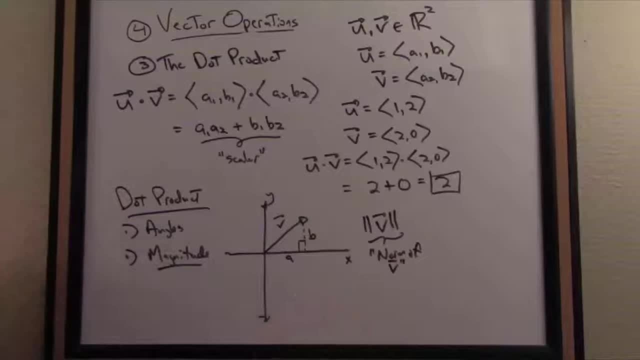 I'll leave off the subscript, so I'll just say the components are a and b respectively for v, and the x component's a, in other words, and the y component's v. How do I find the length or the magnitude of that vector? 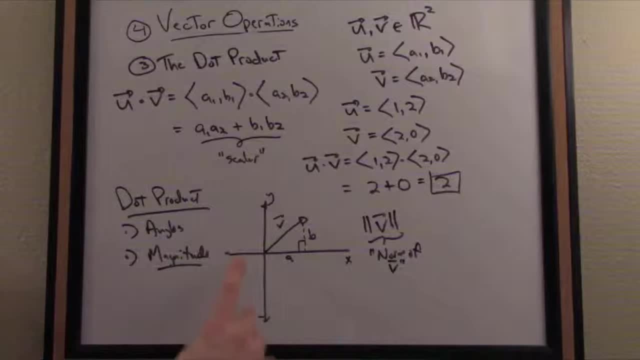 the norm of the vector. Well, simple case of geometry. I've drawn this right triangle encompassing v. so the length of that long edge, or the hypotenuse of the right triangle by the Pythagorean theorem, is just gonna be the square root of the sum of the squares. 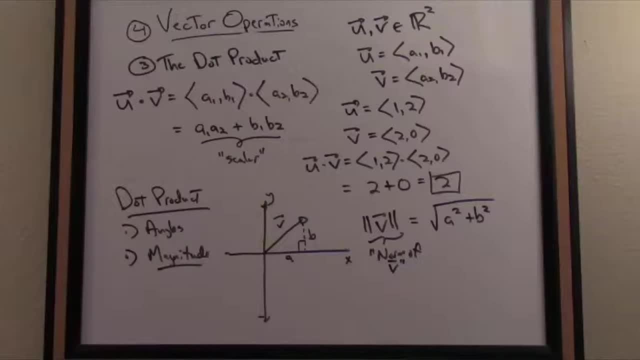 of the components of that vector. right? We've all heard of a squared plus b squared equals c squared. Well, here's the result. equivalently for vectors. So there is the norm, or the length of a vector. okay, I just wanna show you how that connects then. 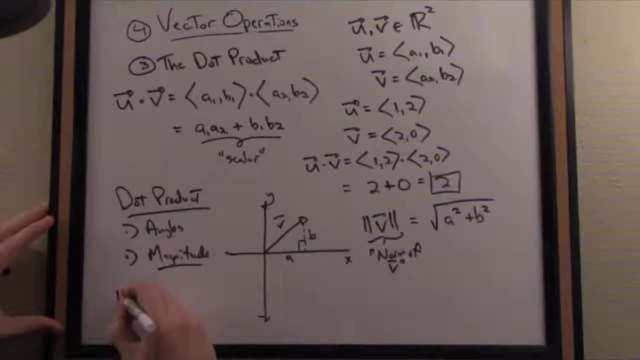 with the dot product. So there's a nice identity. I'm just gonna write here that the norm of a vector squared is equal to the dot product of that vector with itself. So how do we see that from this definition? Well, here's the definition of the norm. 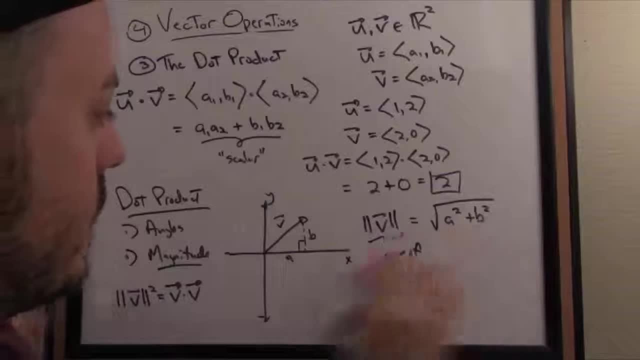 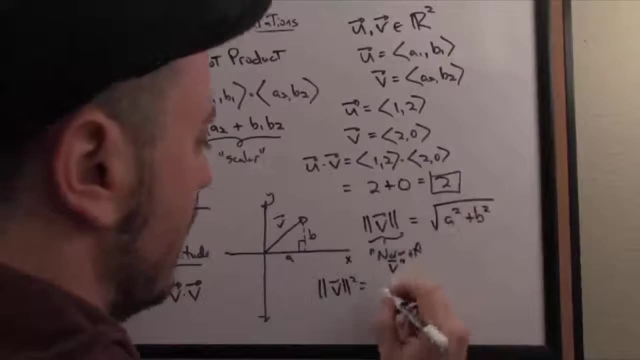 here's the definition of the dot product. Now, if I square both sides of this equation here, what do I get? Well, the norm of v, quantity squared by definition, when I square a square root right, they undo one another, they're inverse operations. 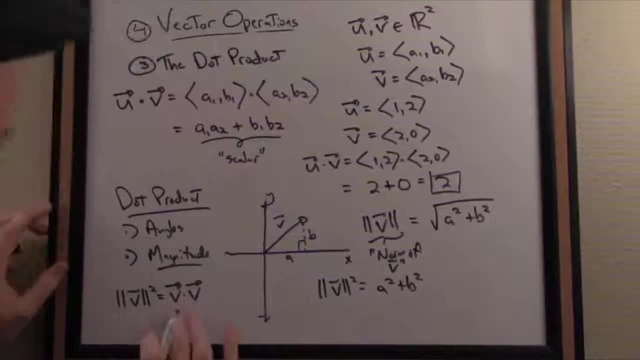 and I just get a squared plus b squared. Well, let's just sort of test the metal here. If I dot v with itself, right by definition, I get a square root of a vector squared by definition. and I get a square root of a vector squared by definition. 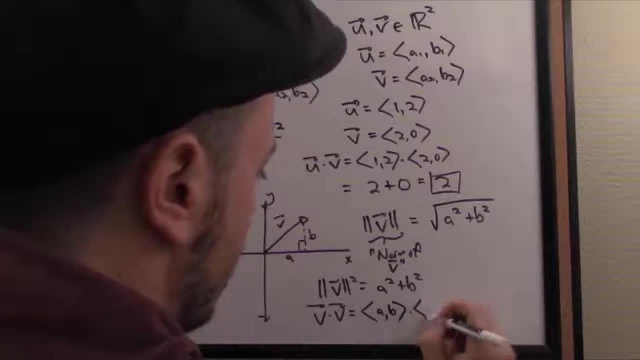 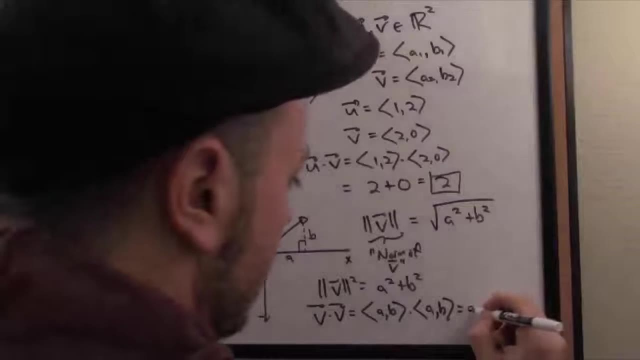 that's like saying a, b dotted with itself a, b. What's the definition of my dot product? I multiply component-wise and then add the products together and you'll notice I get a times a is a squared, b times b is b squared. and sure enough, yes. 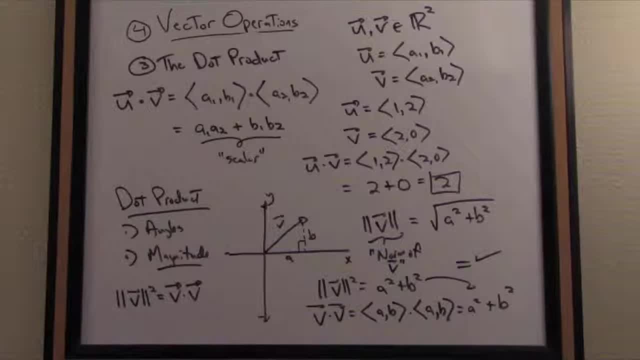 those do indeed match up. So there's a real nice, quick result from the dot product, relating it to the magnitude of a vector. So once again, here's a nice, very common identity introduced for vectors. The norm of a vector squared is the dot product. 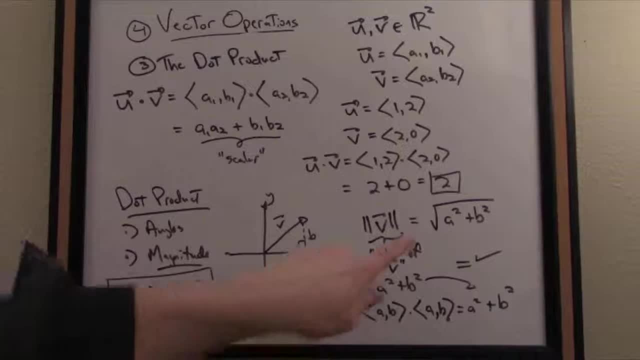 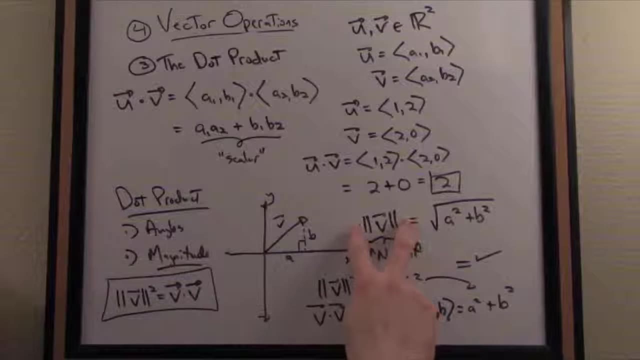 of that vector with itself. and again, the definition of the norm is just the square root of the square of the components of that vector. And one last comment here is if I wanted to extend the definition of the norm or length of a vector to higher dimensions once again. 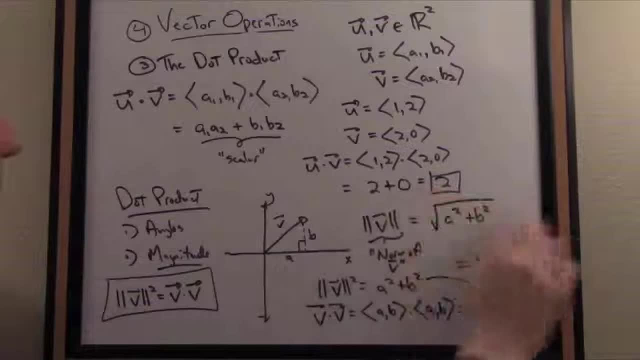 the extension's natural. in mathematics I take the square root of the sum of the squares of all the components. so if there were a z component I would just with inside the radical say plus c squared, if that were the label for that z component. 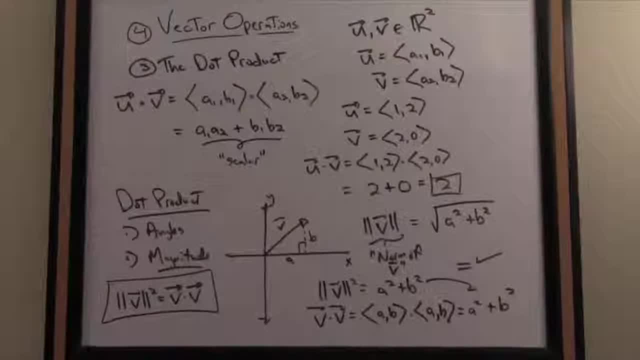 So there we have the basis for the dot product. 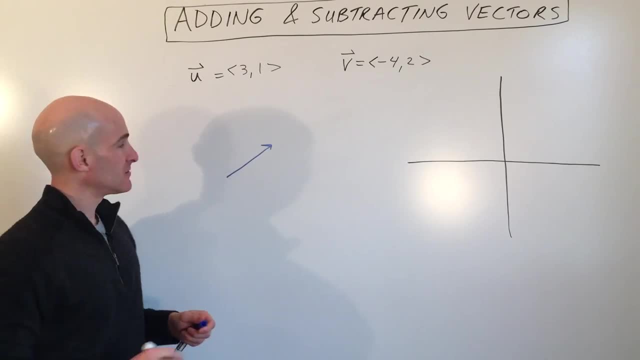 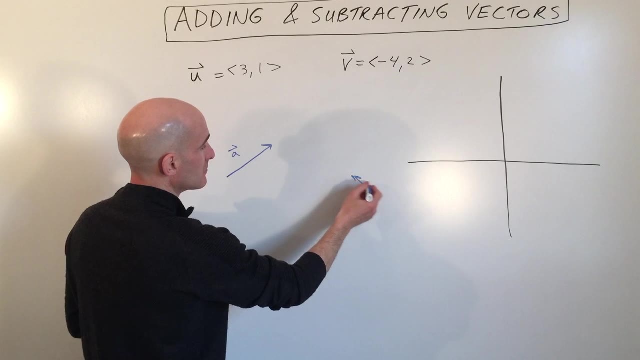 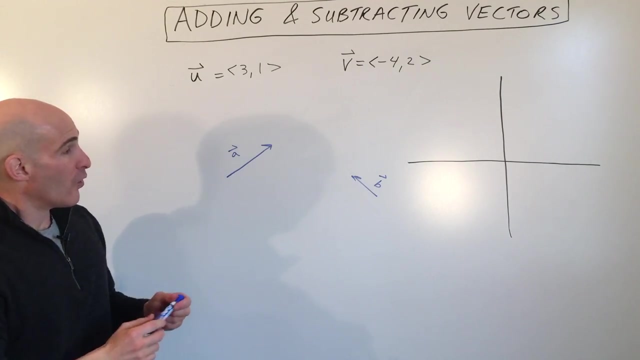 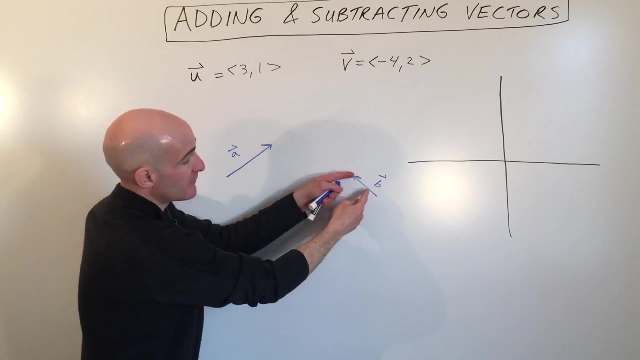 vector like this: okay, we'll just call this vector a, and you have another vector- let's just say it's like this, vector B, and you want to add these together. what you can do is you can take with the vectors, you can slide them left and right, up and down. you just don't want to make the vectors. 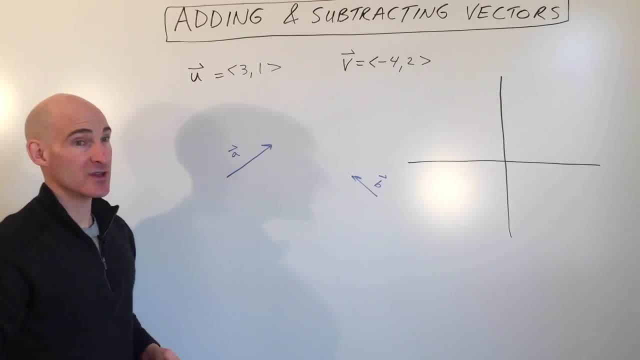 longer and you don't want to change the angle of the vector, because then it would be a different vector, because a vector has a length and direction, so magnitude and direction. but what you want to do is you want to take these vectors and you want to put them in such a way that, where 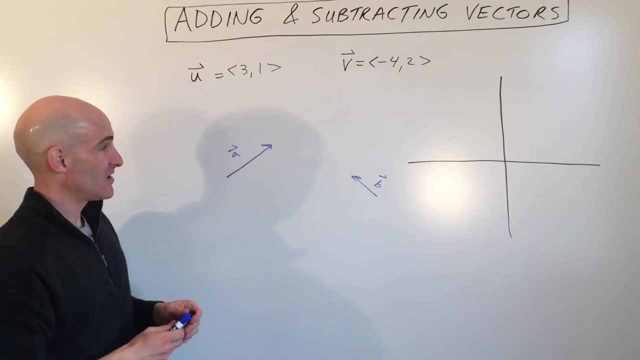 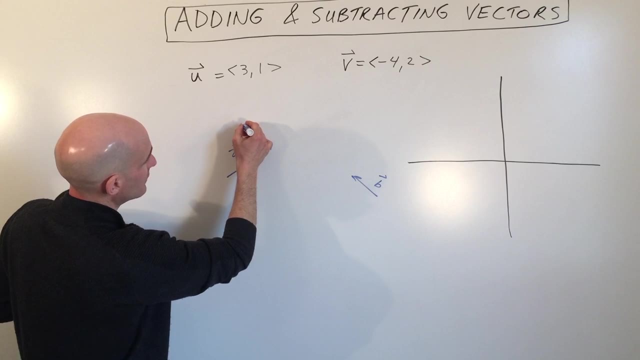 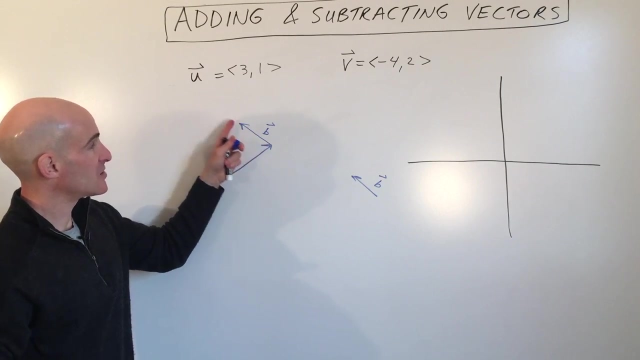 one vector ends, the other vector begins- okay, so what I'm going to do is I'm going to slide this vector over here. okay, keep the angle the same, keep the length the same. okay, there's vector B, so this vector terminates here. the other vector initiates here and terminates there, so the end. 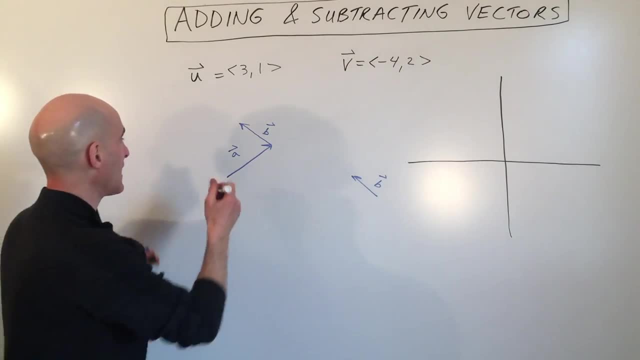 resolved of those two vectors being added together, is this vector right here: a plus B, that's the resultant vector of adding together. so it's kind of like if you were to walk this direction and then walk this direction, the end result is you could have cut through the backyards of your friends and gotten. 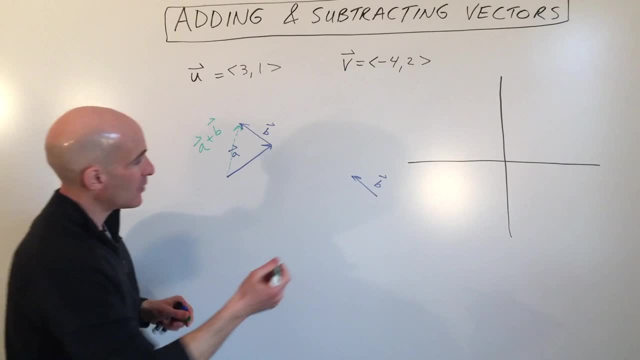 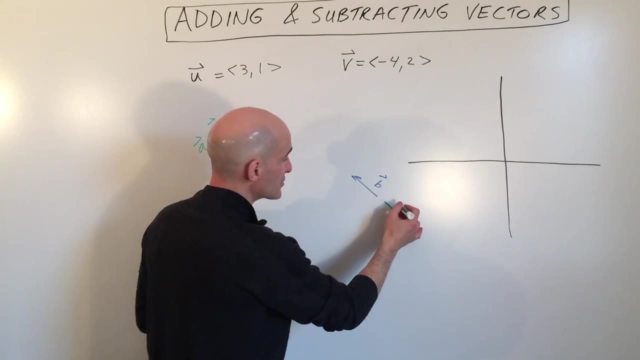 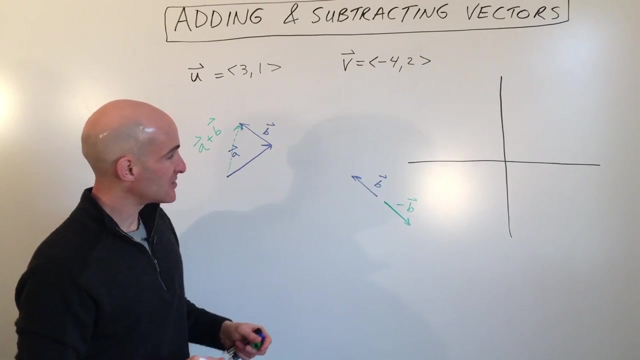 there a little bit quicker. okay now if you subtract vectors. okay, when you subtract a vector, what it means is that the vector is going 180 degrees the opposite direction. so this vector here would be negative. B: same length, 180 degrees opposites pointing the opposite direction. that's a negative.